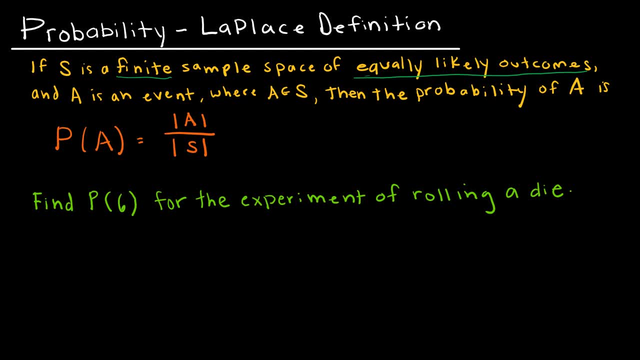 means that it's countable. it ends, it's not infinite. Sample space is all of the possible outcomes. So, for instance, when I roll a die, the possible outcomes are one, two, three, four, five, six. That would be s the sample space. A is an event where a is one of the events that 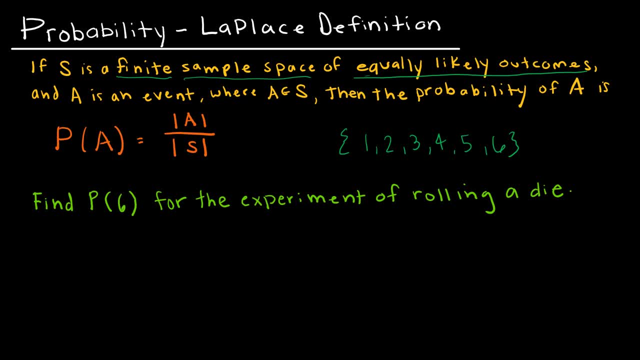 belongs to the sample space, Then the probability of a is the number of elements a over the number of elements in s. So, for instance, if I'm looking at the probability of six for the experiment of rolling a die again, we write it p6 and that just tells us. 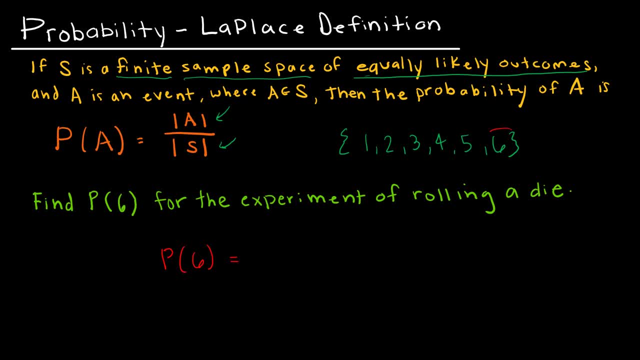 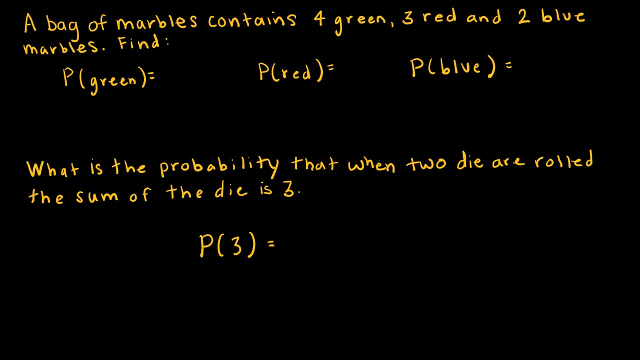 that six is the outcome that we're looking for. One of my items is a six out of six total in the sample space. So I want to look at a few more examples with you, And first I want you to notice that my very first example to you actually doesn't have anything to do with Laplace's. 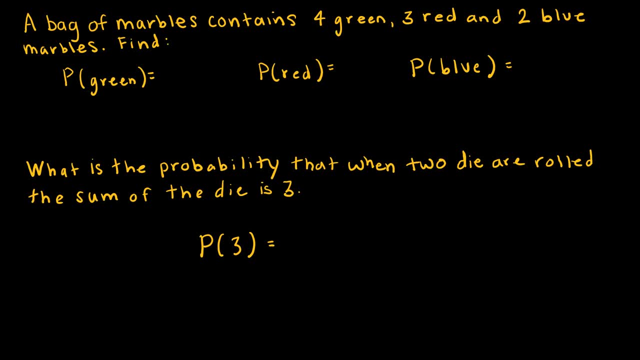 definition, because they're not equally likely. And yet the concept is the same, and we'll formalize that in our next video. But we're saying here that we have a bag of marbles that contains four green, three red and two blue, And so again, I have nine total: four plus three plus two. 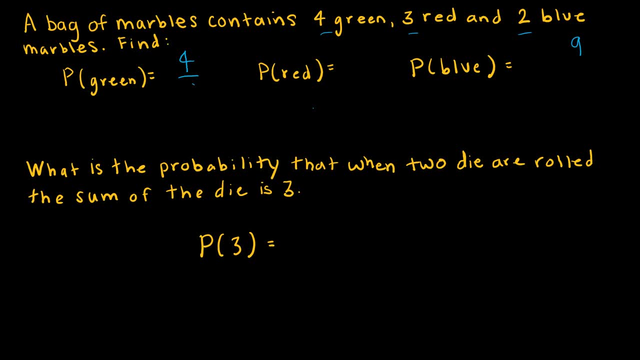 So the probability of a green is that I have four out of nine, The probability of red is three out of nine, and I of course can reduce that- And the probability of blue is two out of nine. So again, that's pretty straightforward and easy. 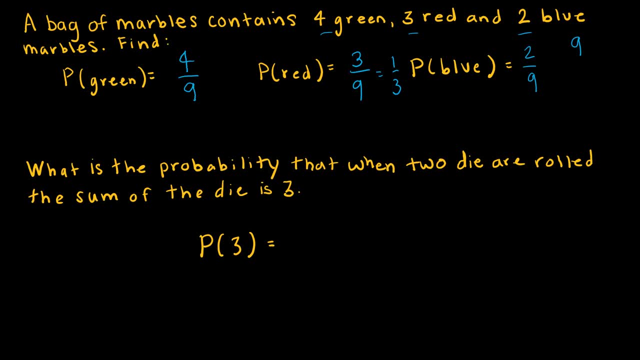 Another, somewhat harder question has to do with the probability: when I roll, two die. So this one's just a little bit harder than the last, but we're saying what's the probability? that when you roll two die, the sum of the die is three? 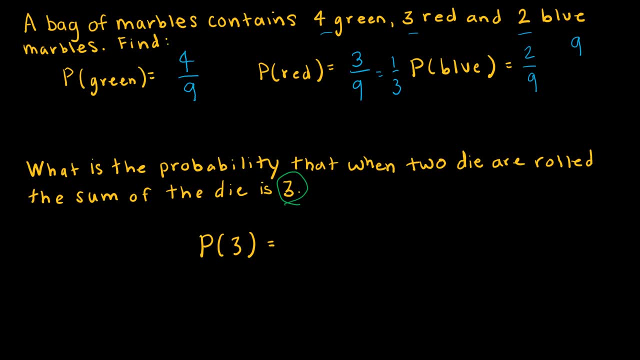 So I know to roll a three, then I have to take get a one and a two, but I can also get a two and a one, So there's actually two outcomes. How many total possibilities are there? Well, I'm rolling a die that has six sides and another die with six sides. 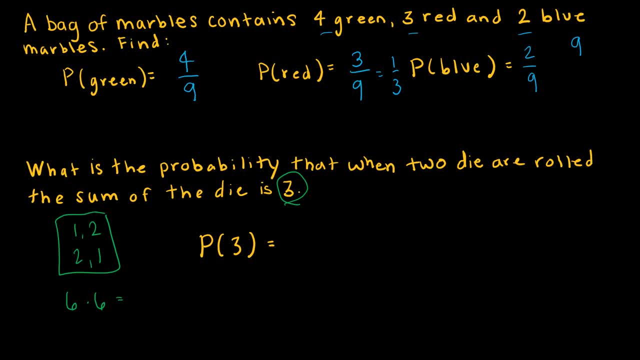 And so, based on our last lessons, where we talked about the number of items, six times six is 36.. That means there's 36 different ways that I can roll two dies, keeping in mind that some of them are going to be like this, where they're. 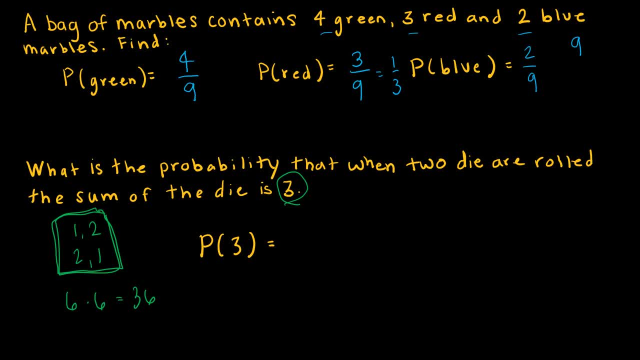 essentially counted twice, but one is the first die and one is the second die, so it's a one on the first die and a two on the second die, or a two on the first die, a one on the second die, etc. so this would be 2 out of 36 or just 1 out of 18. 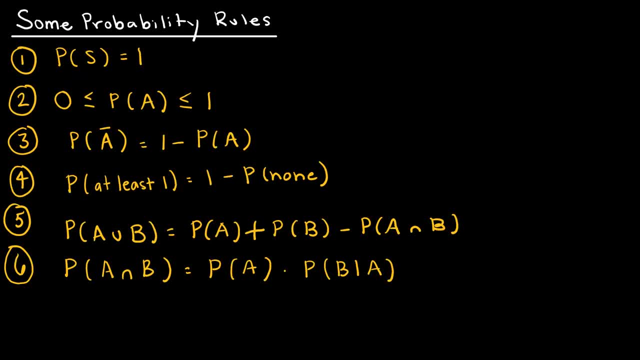 so I want to look at some of the probability rules with you, and some of these we'll, you know, talk about in more detail on this video, and some we will talk about in more detail in the next video. but I wanted to put them all on one side for you just for easy reference. so some of the probability rules and you. 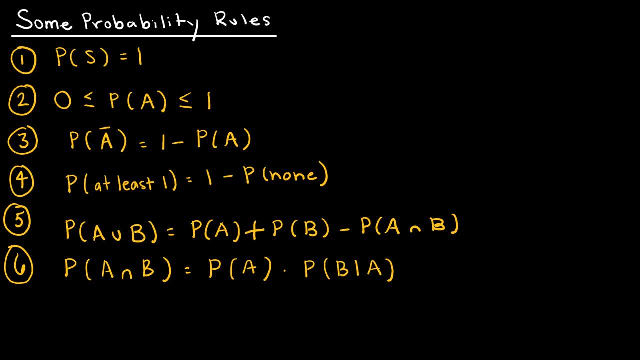 are probably familiar with all of these. so number one is: the probability of all events in the sample space is equal to 1. that one's pretty straightforward. we know that probabilities- and this is rule 2- have to be between 0 and 1, and that 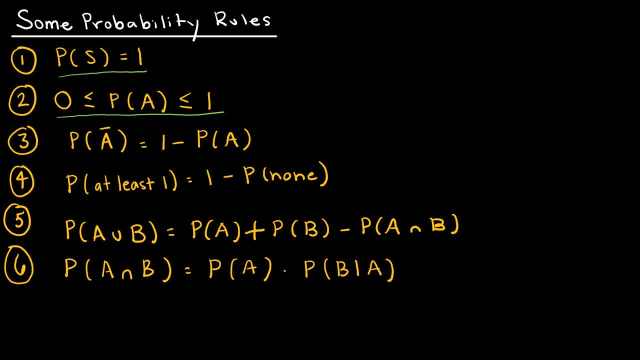 means each and every one of them has to be between 0 and 1, and that means each and every one of them has to be within 1, but the Real Yup. Every event has a probability between 0 and 1, but the sum of all of the 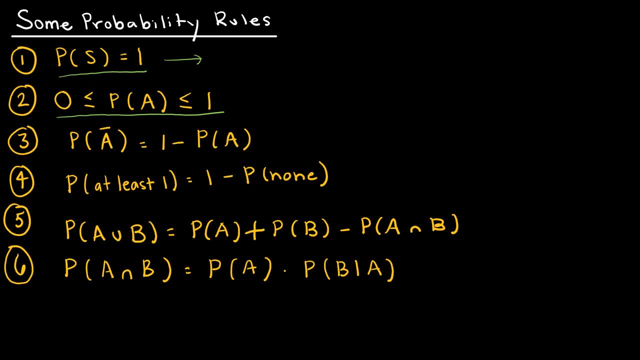 probabilities of events in a sample space have to add to 1. so, for instance, when I flip a coin, I have heads and tails and I know that the probability of heads is 1 half and the probability of tails is 1 half, and then the probability. 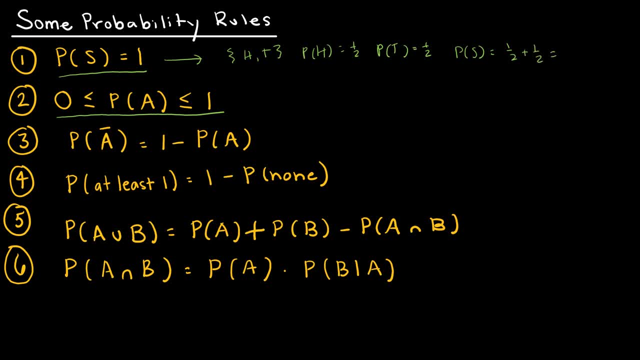 of the sample space, which means all of the outcomes, there is 1, 3 plus 1 half, So it will always work out that the probability of all of the items in the sample space is 1, and that each individual probability then has to be between 0 and 1 inclusive. 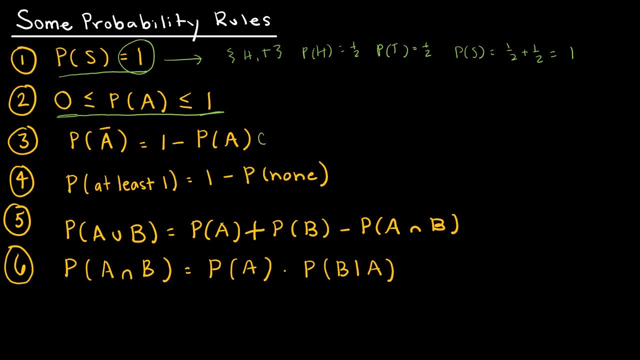 Number three is called the complement rule, And all of that is saying is that sometimes it's easier to do the opposite problem. So, for instance, let's say I wanted to find the probability that I don't roll a 3. So this one, again, is pretty easy to do just on your own either way. 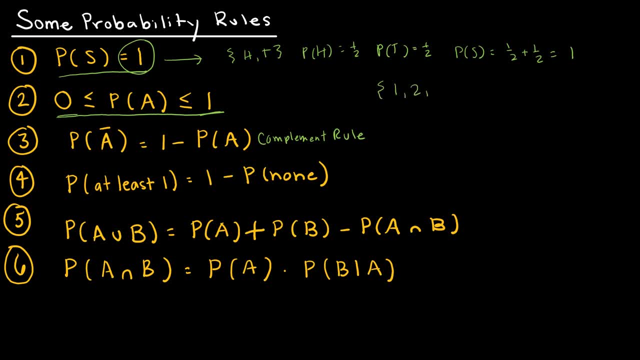 So I know when I roll a die it's going to be 1,, 2,, 3,, 4,, 5, 6.. So I could say the probability of not 3 is 1, 2,, 3,, 4, 5.. 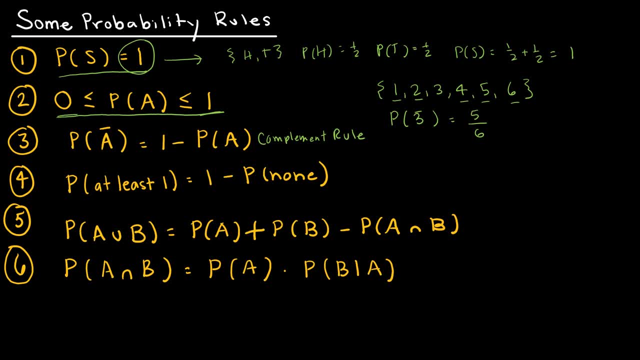 Out of 6 total, And that certainly works. And in this case it's just as easy to do it this way as to use the complement rule. What the complement rule says is, let's say, I know the probability of a 3.. 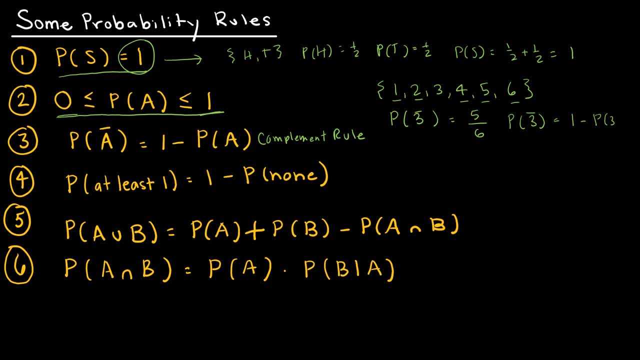 I can take 1 minus the probability of a 3, and that's going to be the probability of not 3.. So probability of not 3 would be 1 minus 1 sixth, which is 5 sixth. So it's 5 sixth. 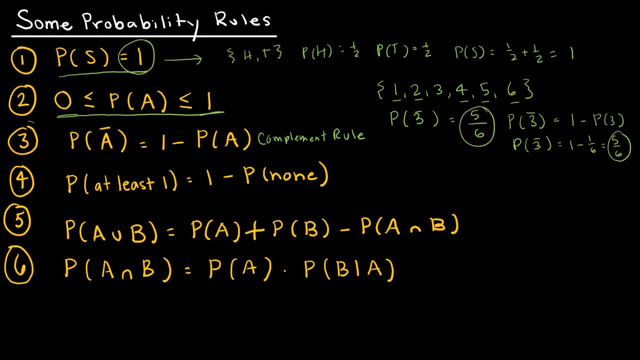 Either way, as we can tell. But again, sometimes it's easier to do the opposite problem, using the complement rule, For instance. let's look at my next example, where I am looking at the probability of at least 1.. And that is always 1 minus the probability of none. 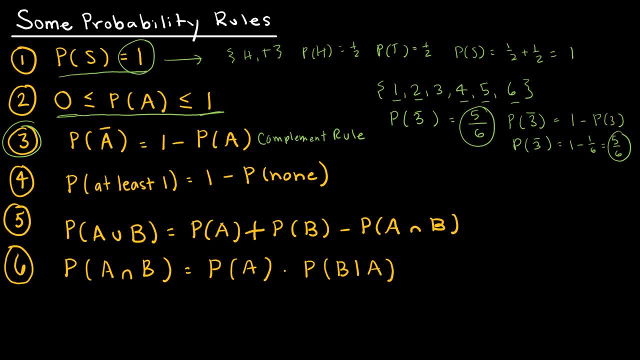 So this again is an opposite problem or complement rule question. This is just a very specific one. So let me give you an example. Let's say I'm rolling Or I'm flipping a coin 3 times And I want the probability that I get at least 1 heads in 3 rolls. 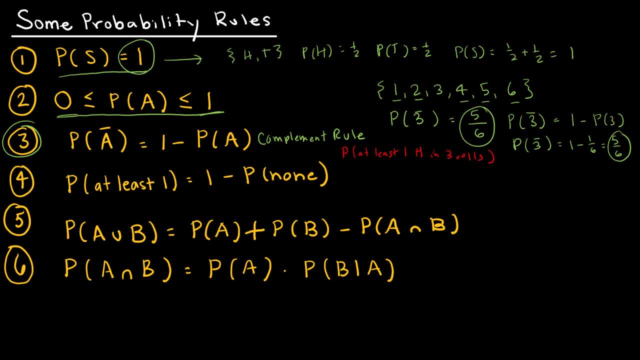 That's my goal Now. if I'm not using this, then I have to figure out all of the different ways. I could Not rolls. I'm sorry that should be flips. I'm getting confused with my die and my coins. 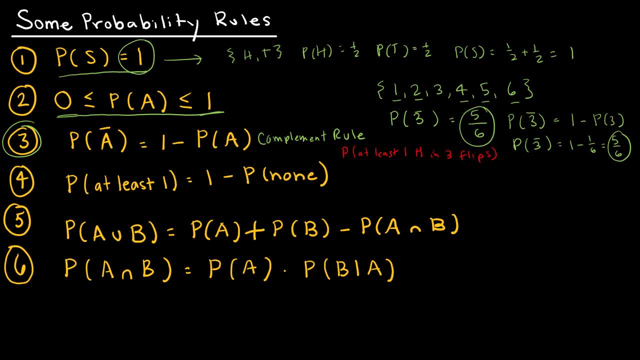 So at least 3 flips, And if I were doing it not using my rule, I would have to essentially figure out all of the different ways that I could possibly flip 3 coins. So I have heads, heads, heads, Heads, heads, tails. 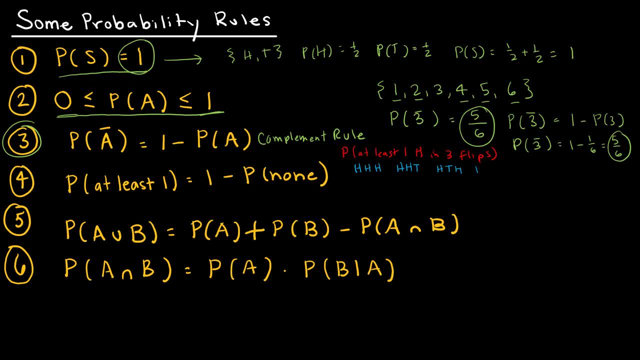 Heads, tails, heads, Heads, tails, tails, Tails, heads, heads, Tails, tails, heads, Tails, tails, tails, heads, Tails, tails, tails. So there's 8 different ways And, of course, if I was just looking for the number of different ways, and we'll talk about that when we get to 6.. 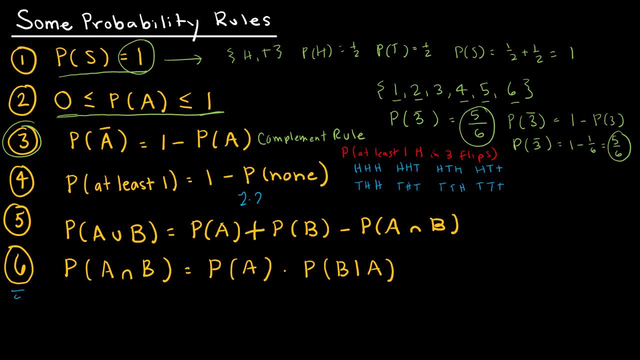 But there's 3 events happening and there's 2 outcomes each time. So 2 times 2 times 2 is 8.. Or 2 to the 3rd is 8.. So- and notice that's how many outcomes I came up with- was 8.. 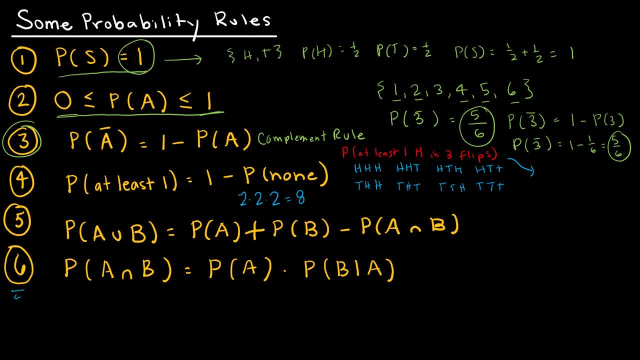 But if I were doing this not using the rule, I would get 8.. So if I were doing this not using rule 4, there I would say: well, let's see If I'm getting at least 1 heads. that's 1,, 2,, 3,, 4,, 5,, 6, 7 out of 8.. 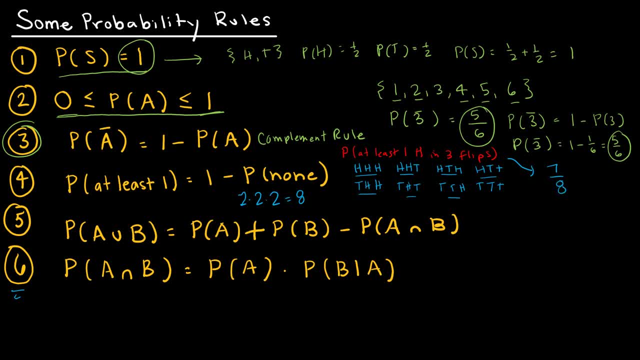 But this rule says: instead of doing it that way, it's easier to say what's the probability that I get no heads, which is just this guy Tails, tails, tails, Tails, tails, tails. And so then I could say that this probability is 1 minus 1 out of 8, which again is 7 out of 8.. 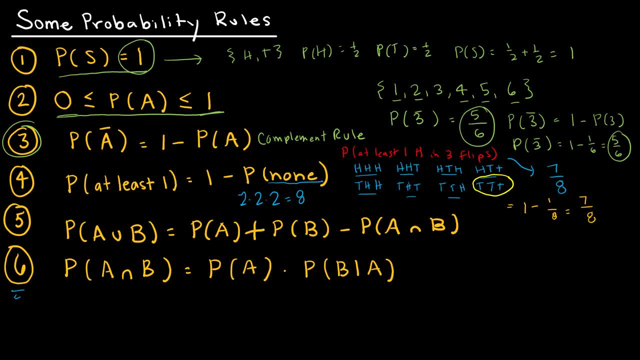 So I end up getting the same answer, but again, it's just another way to go about it And quite often when you get an at least, it's going to be way easier to do it this way. Rule 5 has to do with when I have only one event occurring, but I have more than one outcome. that's okay with me. 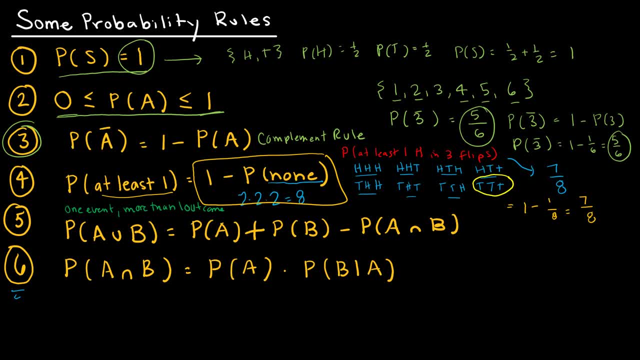 And so, for instance, I'm going to go back to rolling a die. Let's say I want the probability of a 2 or a 4, which means I'm only rolling the die once, But I'll be satisfied if I roll a 2 or a 4.. 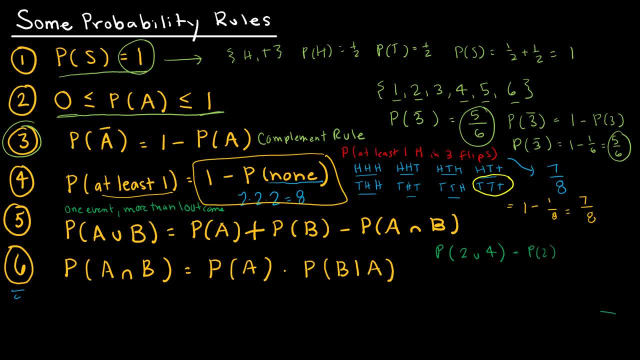 So I would just find the probability of a 2 plus the probability of a 4.. And then this last part comes into play when I have events that are not disjoint. So if I have an overlap, if I could roll a die and get both a 2 and a 4 on the same roll, then I would have to do some subtraction. 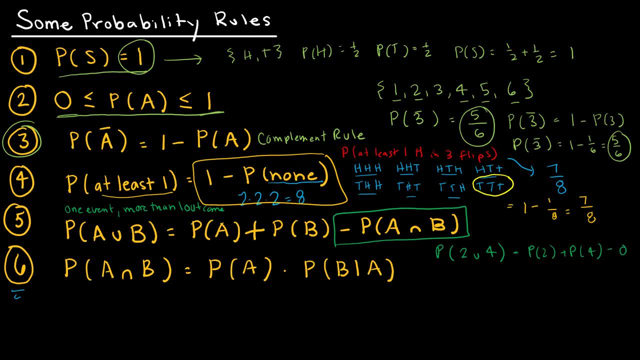 In this case, that's just going to be 0. Because there's no way to roll a die and get both A 2 and a 4, because 2 and 4 are disjoint events, And so what I get here is 1 out of 6 plus 1 out of 6, again plus 0, which is 2 sixths or 1 third.